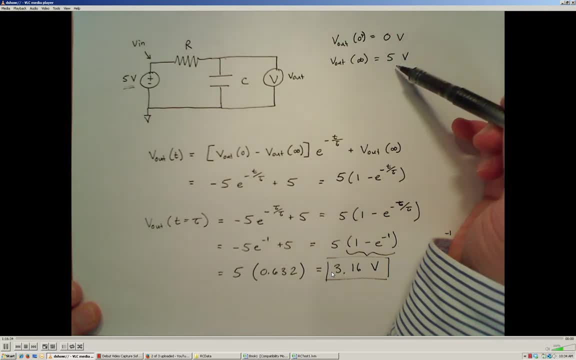 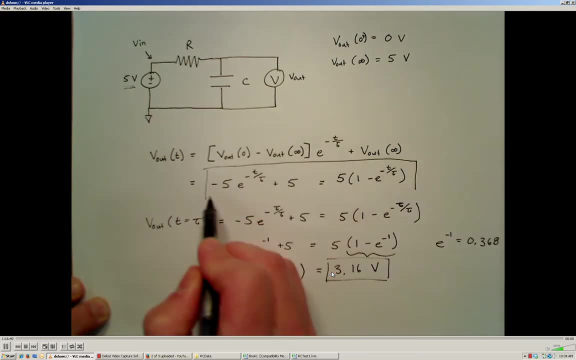 and the final state of the steady state voltage across the capacitor that the output voltage is going to be given by this equation right here. Okay, So I have measured the voltages and I have measured the time t. So now what I want to do is- it's my job- to try to figure out what this parameter. 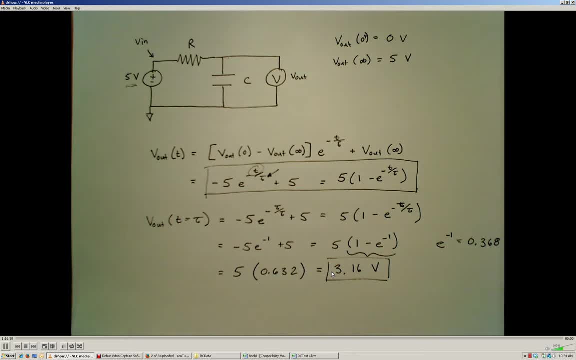 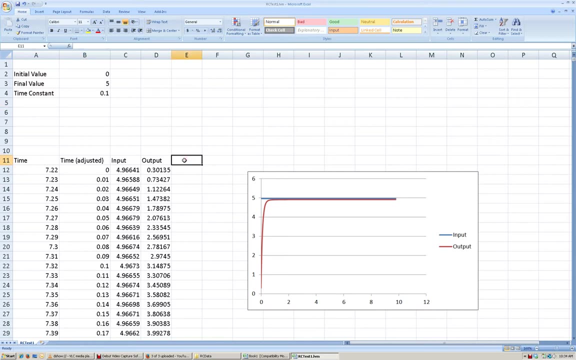 this unknown parameter of the time constant tau is. So what I'm going to do is I'm going to go back to my spreadsheet here and I'm going to create another column that I'm going to call the model. All right, And the model is going to be the equation that we derived. 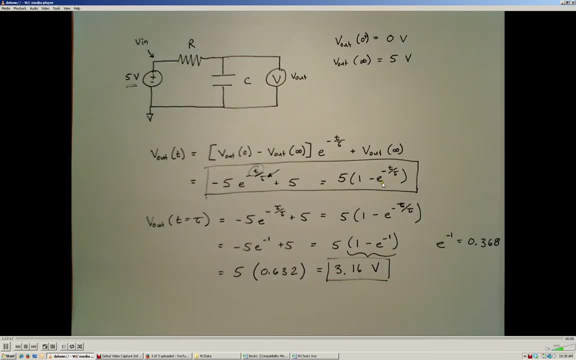 for how the output voltage should change as a function of time. So it's going to be this equation right here, All right Where- and I'm going to use the second form of the equation right here- where 5 corresponds to our Vout voltage. 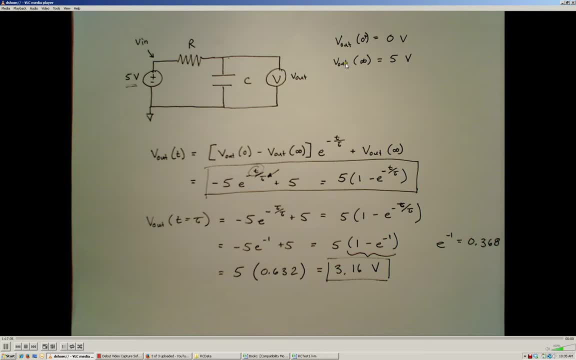 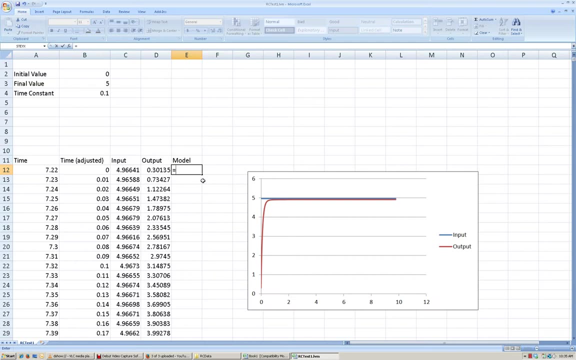 Sorry At the after the. the circuit has been operating for a long period of time. Okay, So I'm going to go back to that, And now my model is going to be- I'm going to reference the final value right here- absolute. 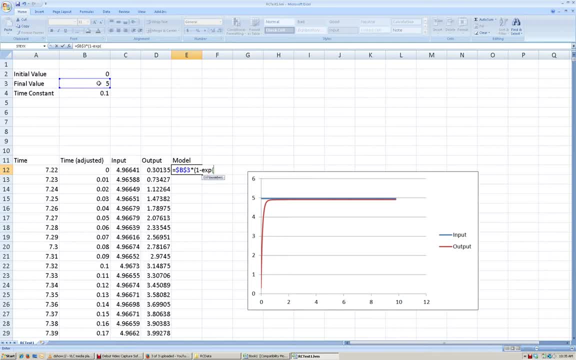 multiplied by 1, minus the exponential function raised to the negative t. So I'm going to reference my adjusted time column divided by, divided by the time constant value that we're trying to determine. Okay, And we know we have estimated that it should be about 0.1.. 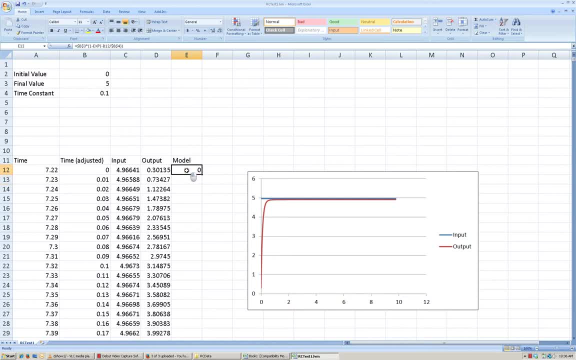 So I'm going to go ahead and enter that and make sure that the time constant value is referenced, absolutely All right. So now in my model, I'm going to fill in my model all the way down And I'm going to add yet another column to my data, and my model is going to be this way. 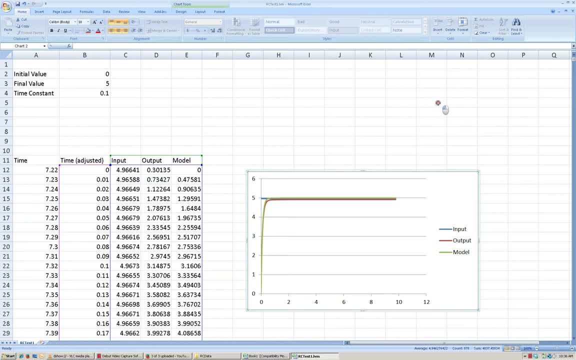 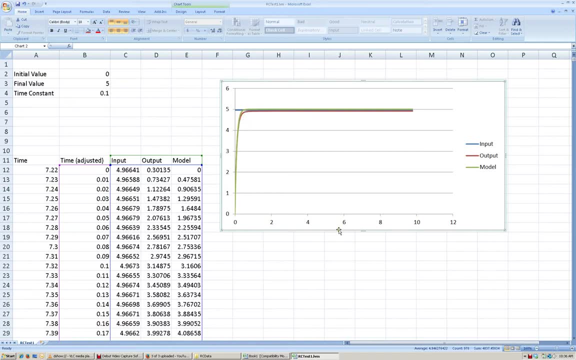 This green line right here, All right, And I see from that now that the estimate of 0.1 is pretty close. but we see in this region right here- let me expand the axis here so that we can see things a little bit better- 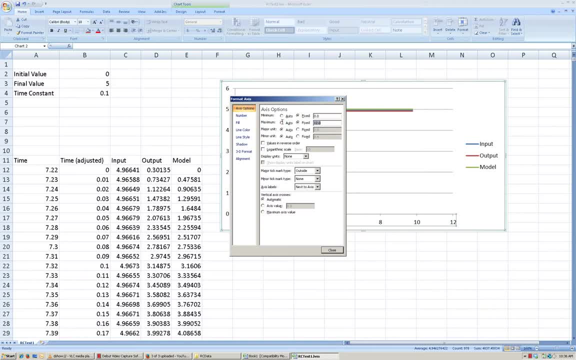 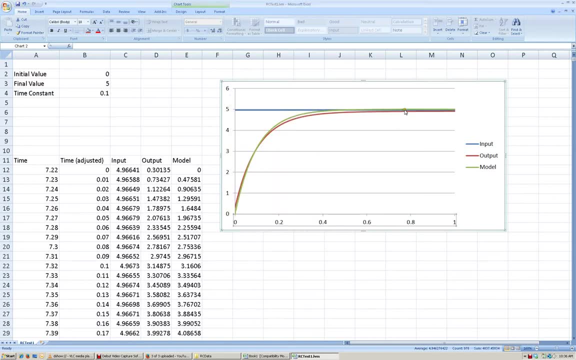 I'm going to go from a minimum of 0 to the interesting things happen all within one second. Okay, So we see that the model fits fairly well to the information, but not not perfectly Okay. So what I'm going to do now is I want to, as best I can, fit the model to the data. 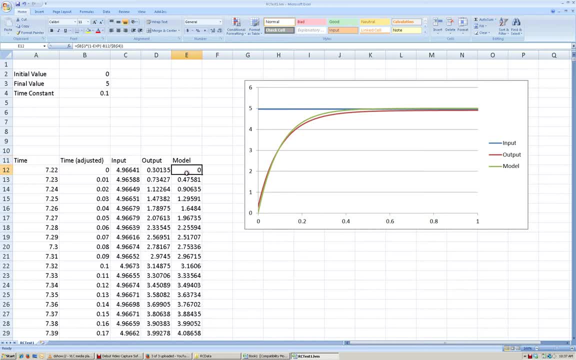 So what I'm going to do is calculate the difference between my modeled output and the measured output. Okay, So this will be the square difference between the model and the measured data. So I'm going to take my modeled output And I'm going to subtract from that the output that we actually measured. 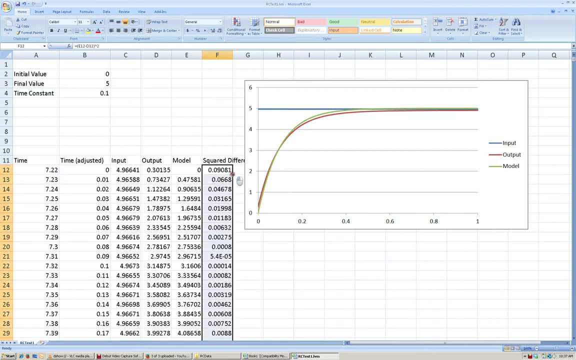 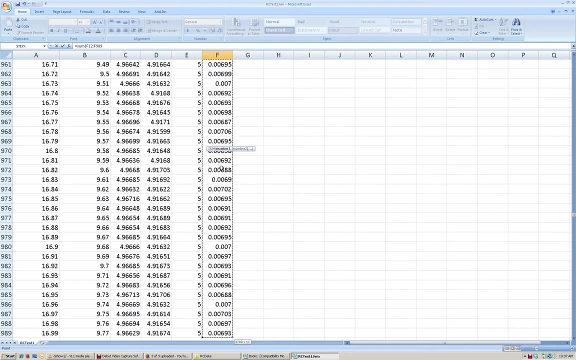 And I'm going to square that for all of the data points that we collected, And then I'm going to take that entire column and sum up all of those squared differences. All right, So I'm going to take the sum of all of that data. 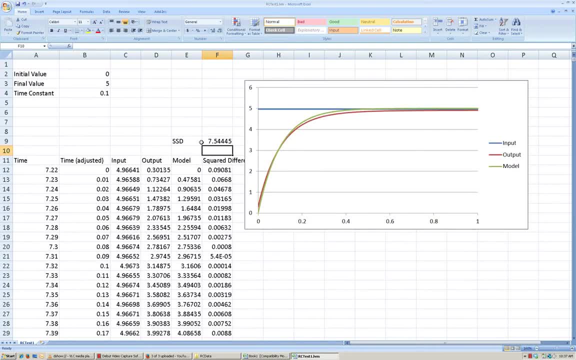 All right, And what we're going to do now is we're going to use the solver To um try to minimize the sum of squared deviations based on uh by adjusting the time constant value. Okay, So, uh, I'm going to go over to my data column. 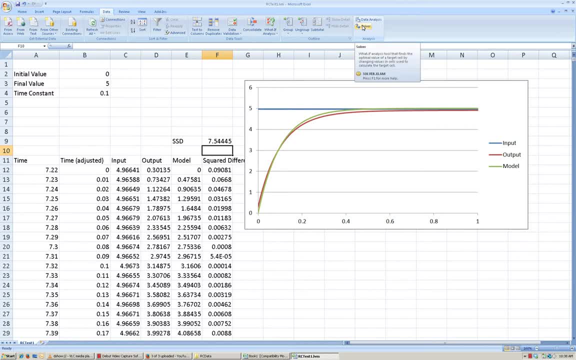 And I should have the solver tool enabled. I'm going to click on the solver tool. It's going to ask me what parameters I want to set. So I want to set the target cell to be the um sum of squared deviations, the value of that. 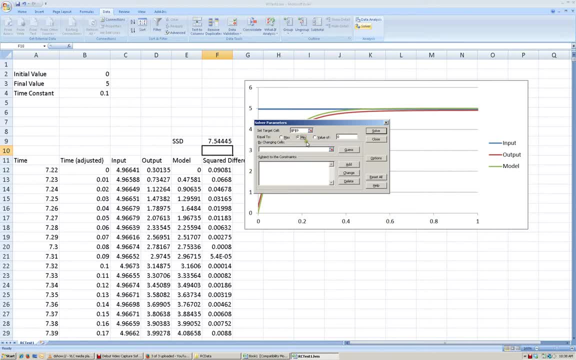 Okay, Okay, Okay, Okay. So I want to minimize that. So I want to set it equal to minimum And select the cells that I want to change. Right now, I'm just going to change the time constant cell. Okay, After all of that is entered, we'll click the solve button and see what it comes up with. 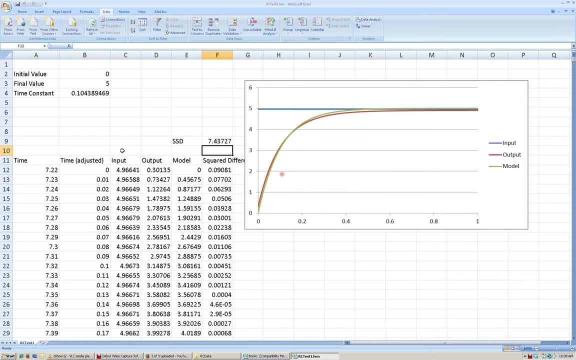 Okay, And what it came up with for the solution here was that the time constant is .104 seconds, Which is very close to what we had, But it's a better estimate, Because now we're using all of the data, uh that we acquired to estimate that. 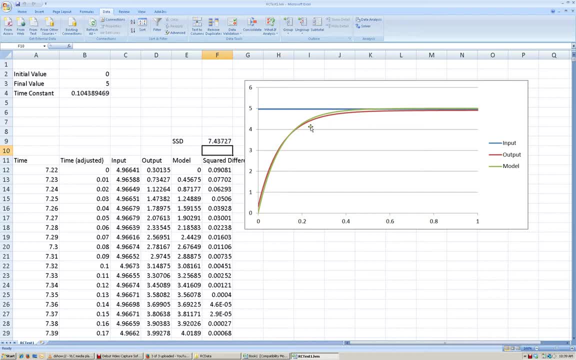 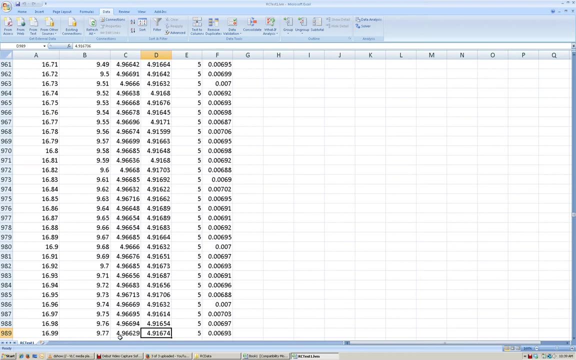 Now, one thing that we also notice is, um, in this, uh, in our data, the output never fully reaches the 5 volt value. So if we go back to our measured output and we scroll all the way down, we see that, um, our input value was measured as 4.966 volts. 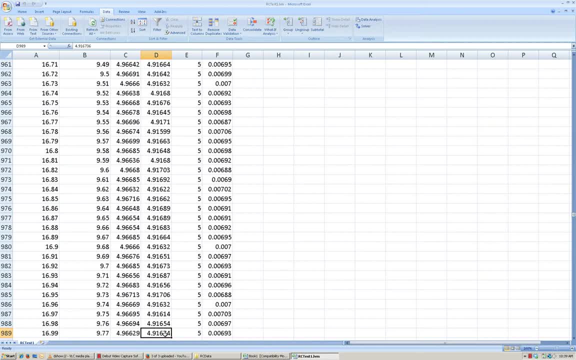 But our output only reached 4.916.. So there's a slight difference between the output and the output. So there's a slight difference between the um st- uh, between the input value and the final steady state value. So, um, we recognize from our measurements a couple of things. 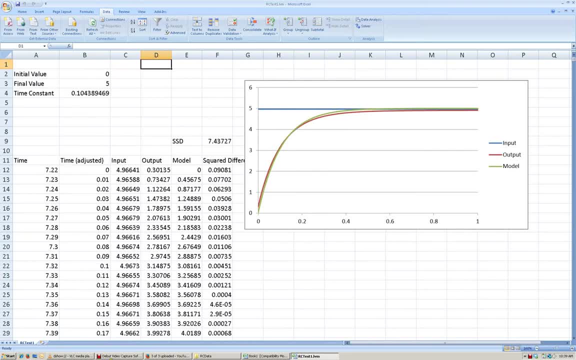 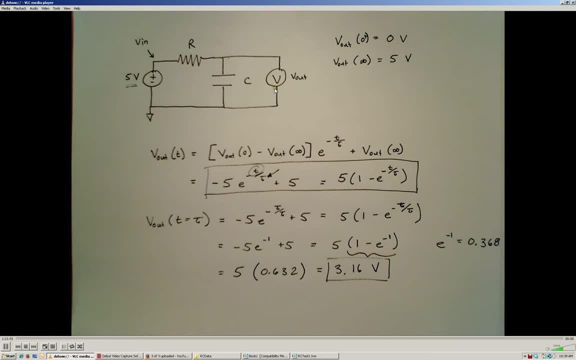 First of all, our output is not ideal, And what that implies is that the um, that this voltmeter, or the uh data acquisition card, is not an ideal data acquisition card. In other words, it probably has some resistance associated. 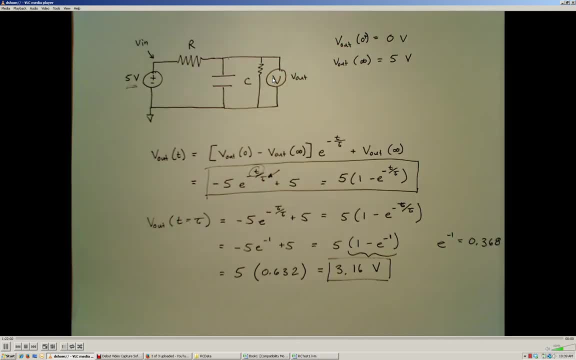 Alright, So we also now can now go back and we can adjust our model and we can readjust the output um, the steady state output voltage, to account for that, And then our time constant is going to be different because our um, because this additional resistance due to the data acquisition card. 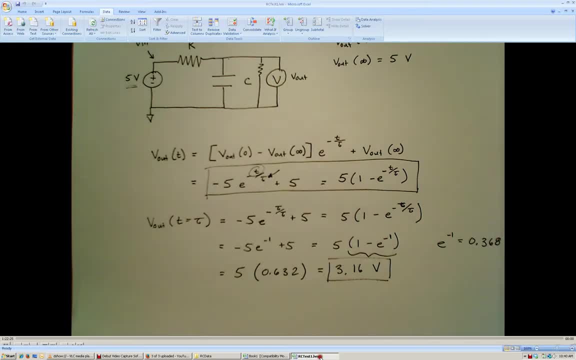 So I can come back to my test information right here And now. what I want to do is I'm going to go back to the data acquisition card, And what I've done here is my equation, And then again I kinda go to the data acquisition card. 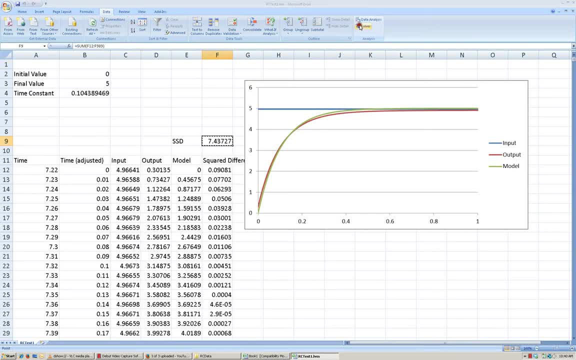 Right, go back to solver. but instead of allowing solver to only change the time constant value, I'm going to allow it to change the final value as well. So I'm going to select both the final value and the time constant and allow it to change. 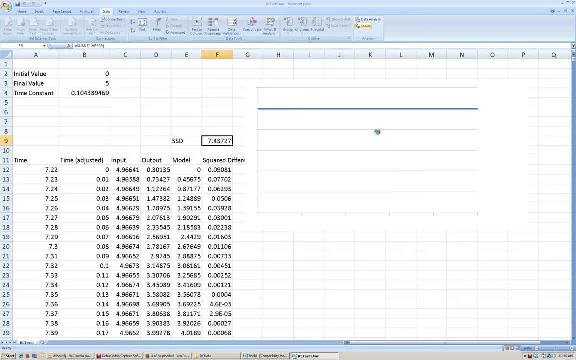 both of them Alright, and we're gonna click the solve button again and see what it comes up with. Alright, and now that we have a solution from the solver, we see now that our model looks very much like our data that we had. So now it. 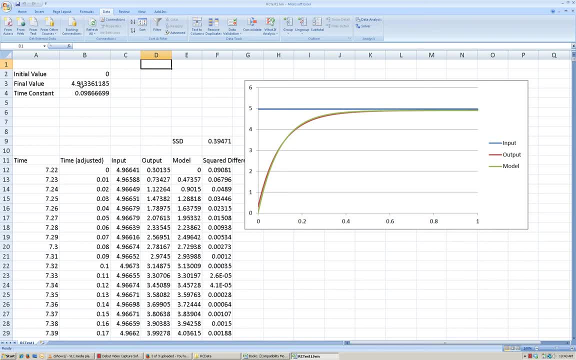 says, the final value or the steady state value should be 4.913,, which is very close to what we measured, And now, because of that, our time constant has decreased a little bit as well. So it's still close to 0.1, but it's actually a. 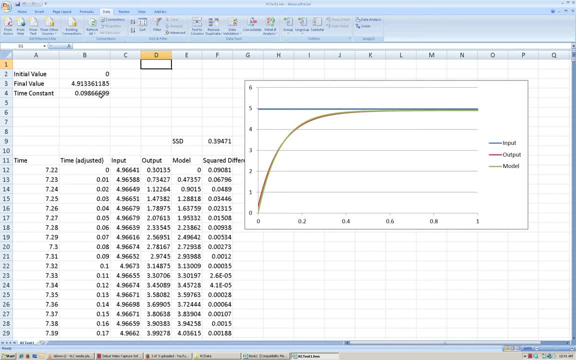 little bit lower than 0.1. now The other thing that we need we can do is we can run, rerun solver And allow it to change the initial value, the final value and the time constant and see if that makes any more sense to us. Now we still haven't described why. 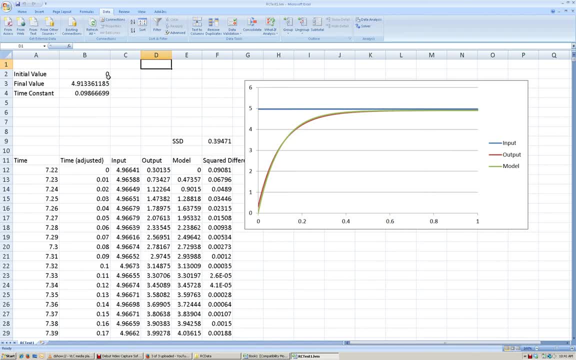 all of this is happening. Let's see, but right now it still says the initial value is best kept at zero. So that, so that's going to give us the best result for the data that we acquired. So, again, what we can, what we have not done, is: 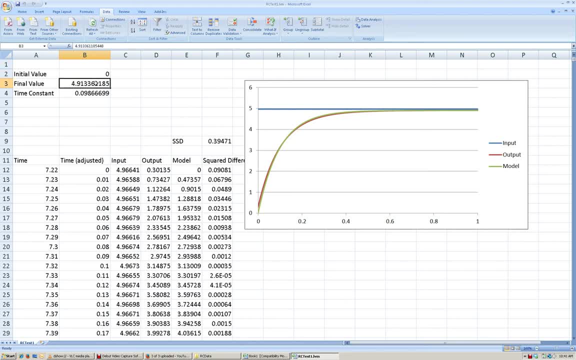 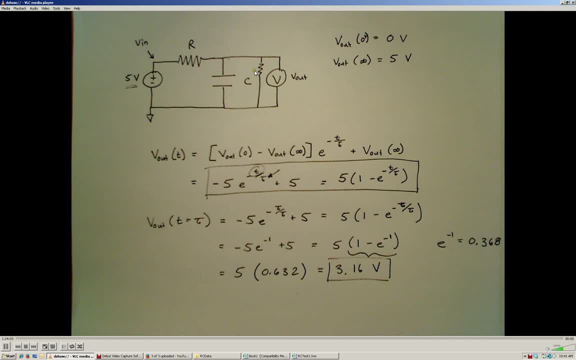 we have not. we don't haven't fully explained why this final value is not reaching the full 5 volts, but we have. we suspect that it's due to this additional internal resistance of the voltmeter or the data acquisition card. Of course this. 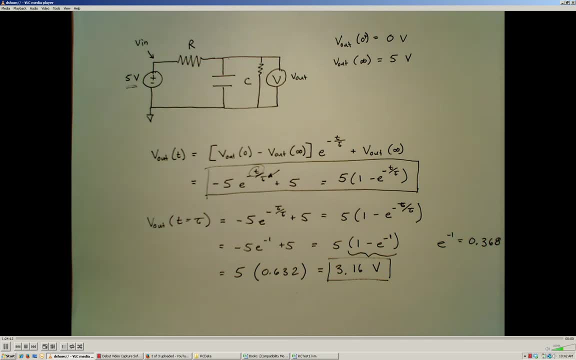 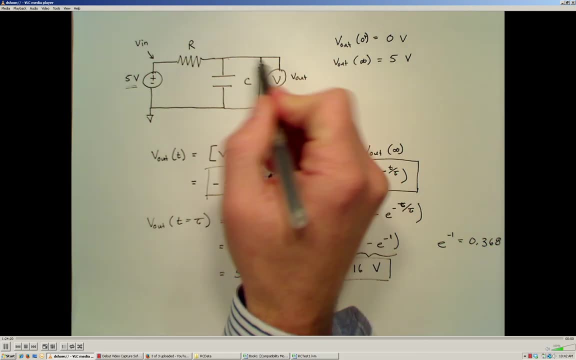 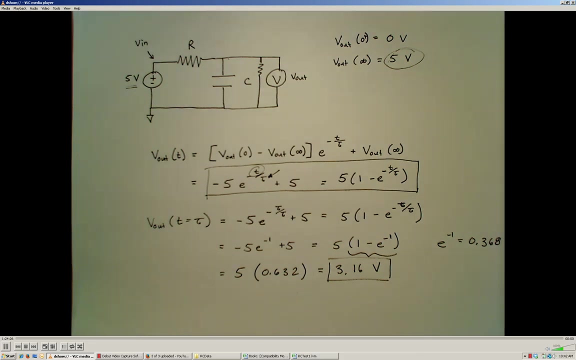 is a different system now, So these equations no longer apply because this is, in steady state, going to act like a voltage divider that's going to reduce the total steady-state voltage across the capacitor. Okay, so those are two different methods that we can use to estimate the time constant.